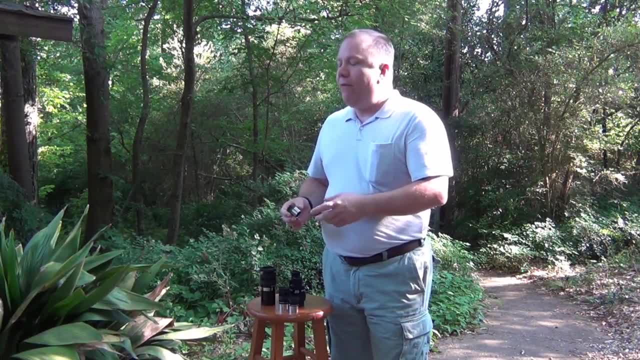 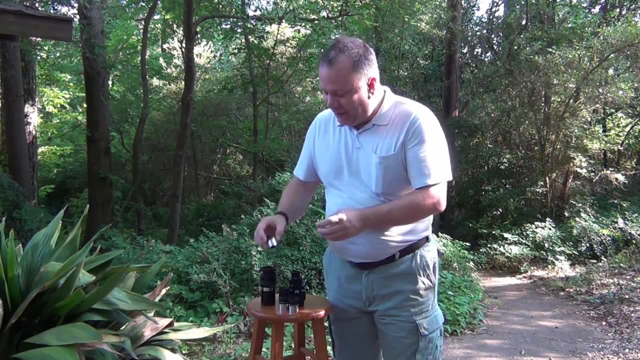 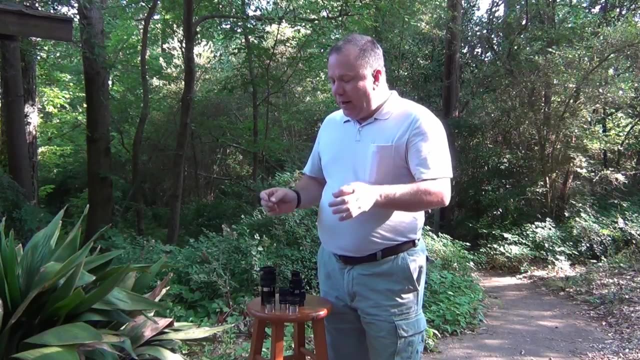 want to get ridiculous. one of the things that I did when I first started out was I got a 6.4 millimeter. I have never gotten a decent image with this. The problem gets to be that, because seeing conditions are never perfect, the higher the magnification, the less clear the object. 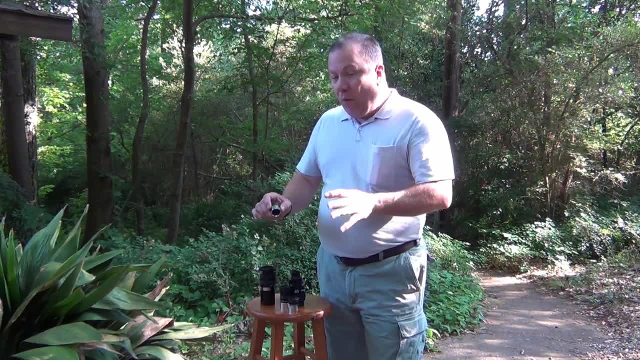 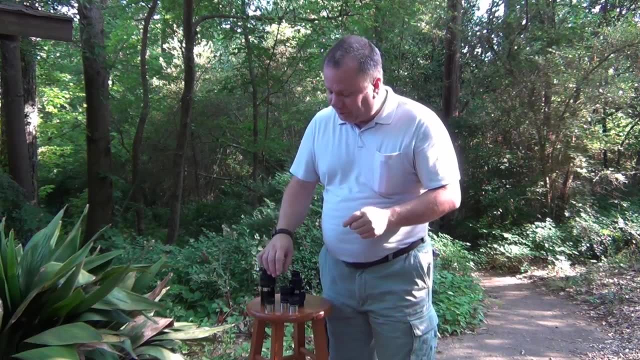 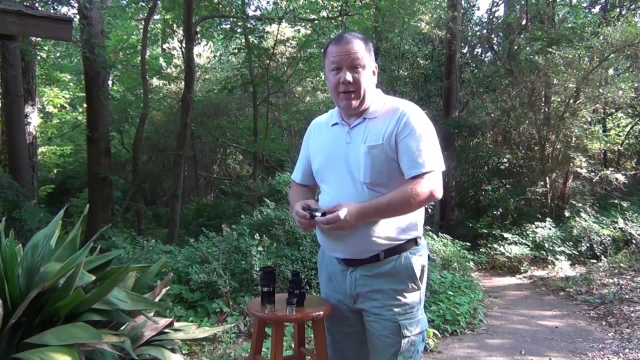 becomes to the point where with this 6.4 millimeter when I pointed at Saturn or Jupiter, I can kind of sort of tell it might be a planet, but not really. 10x I can use more often than that and it gives me a little bit better views. The 25x gives you excellent views but not a lot of magnification. 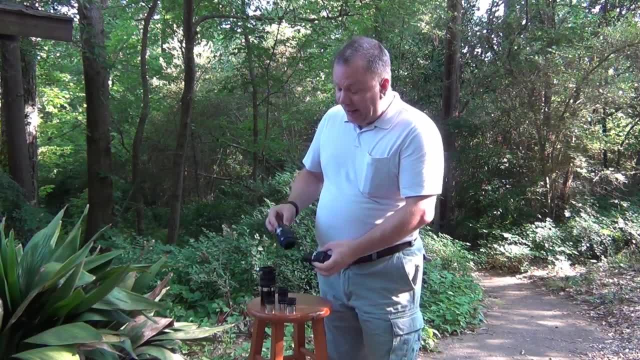 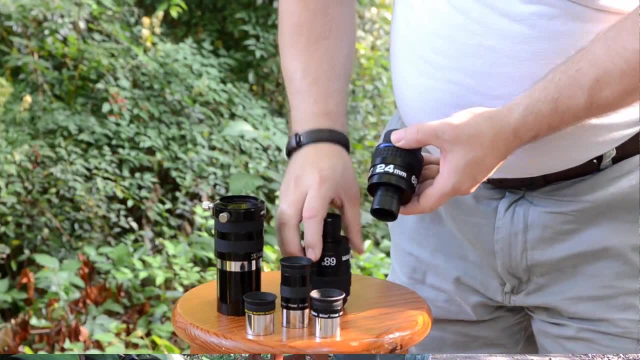 Now, one of the things you may notice is there's some really big eyepieces here. These two are Orion Stratus eyepieces in a 13 and a 24 millimeter. Look at this 24 millimeter, 25 millimeter, Notice how. 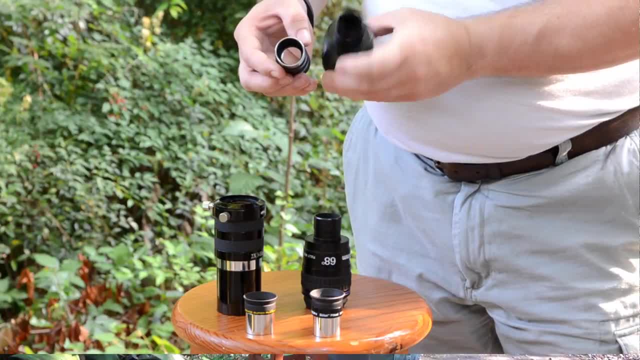 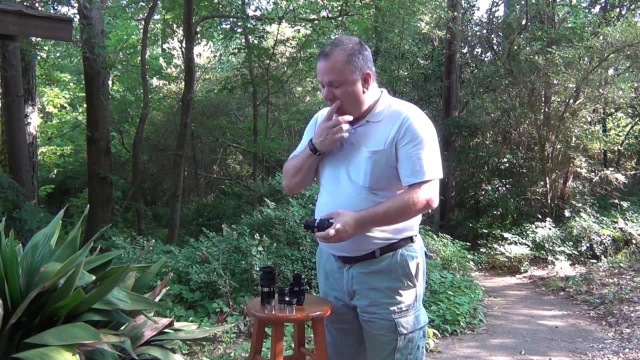 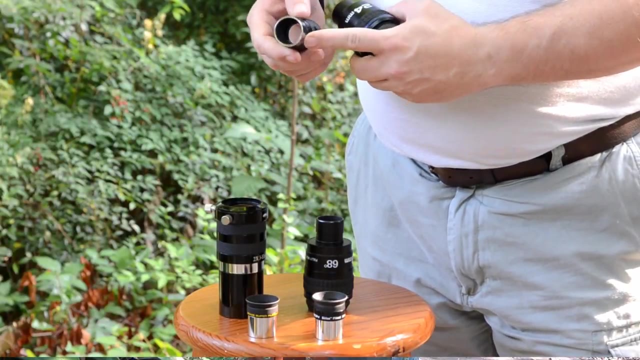 much bigger this eyepiece- the 24- is than the 25.. Why is that? Well, a couple of reasons. First off, there's two different sizes that telescope eyepieces have to worry about. One is this right here. Notice that this and this are the same size. However, up here is another place where 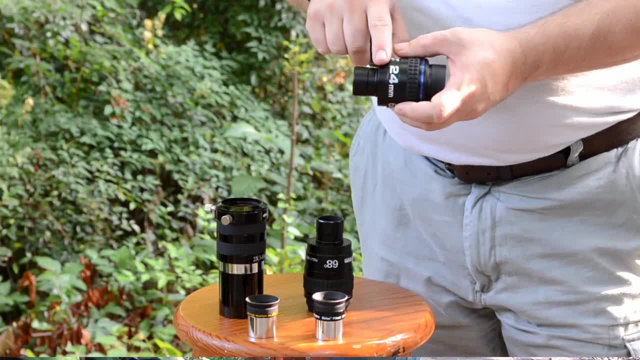 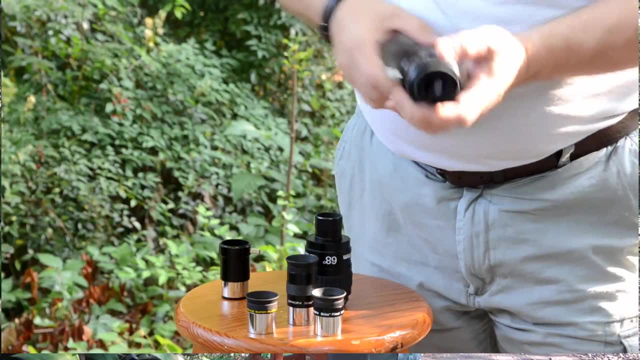 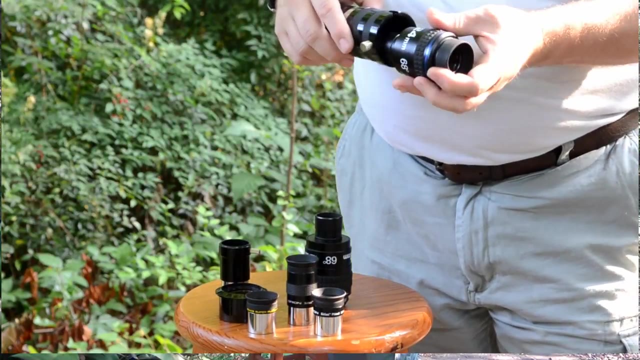 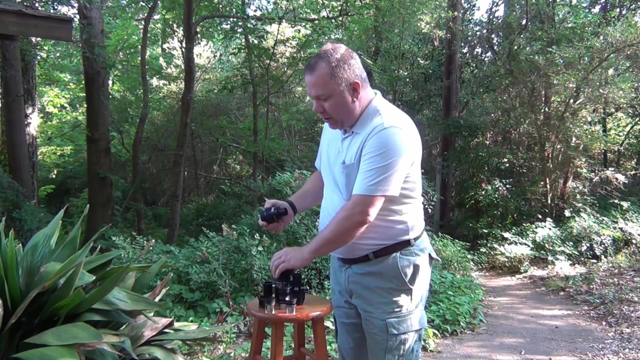 you can mount this telescope eyepiece. So you got one inch and two inch basically, And on your telescope the one inch may fit in like that or, as is the case with this particular adapter, the two could fit in like that. Now, the reason for them being two different sizes and having an adapter is that two inch eyepieces 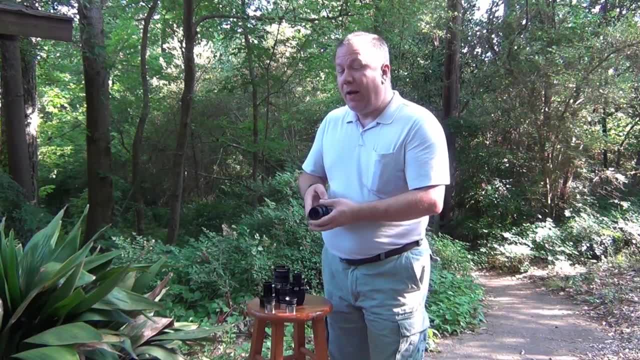 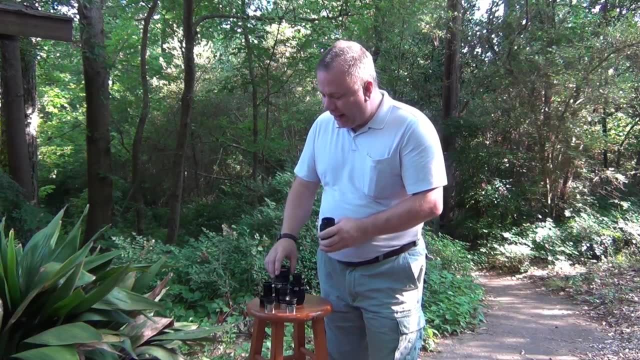 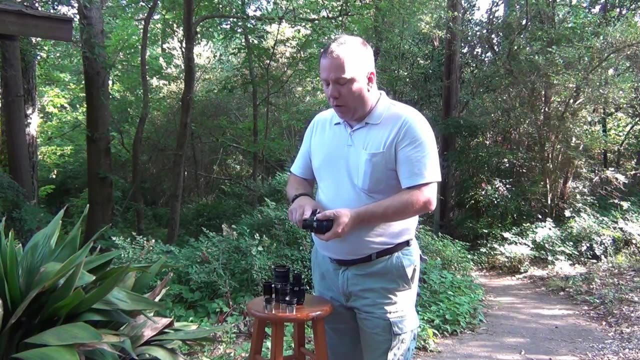 allow you to use larger eyepieces- and we'll see why here in just a minute- that give you greater field of view and greater eye relief. We'll get to that. Smaller telescopes and less expensive ones may only have the small, which is about an inch and a quarter. 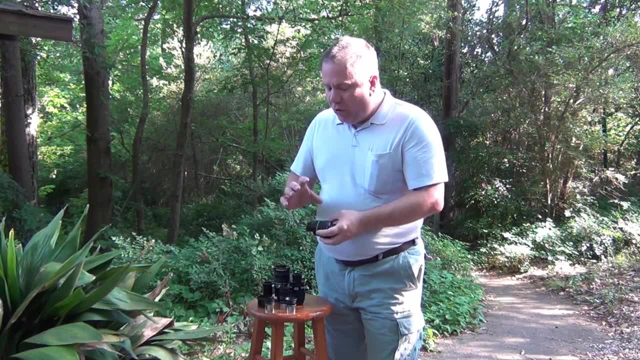 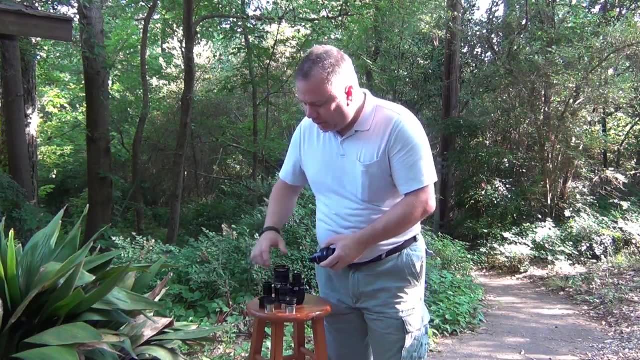 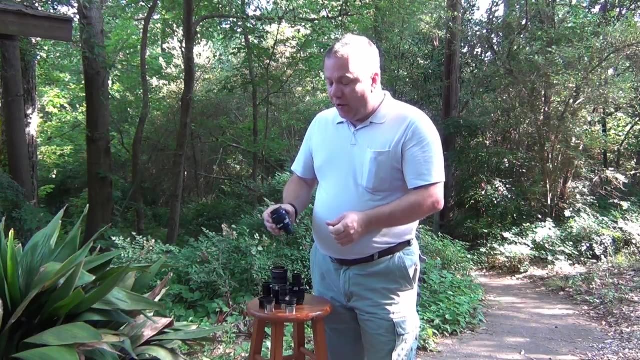 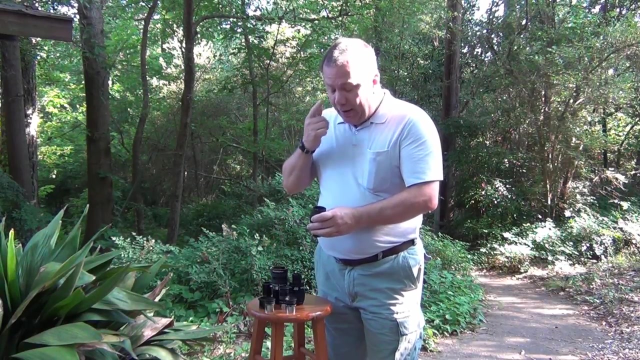 Done, So your higher-end telescopes may have both – two and then an adaptor to take it down to the small one if you want to use it. So one of the things we talked about is eye relief, and that's one of the reasons you use these bigger eyepieces. Eye relief is the distance that you're eye is from here to get a clear. 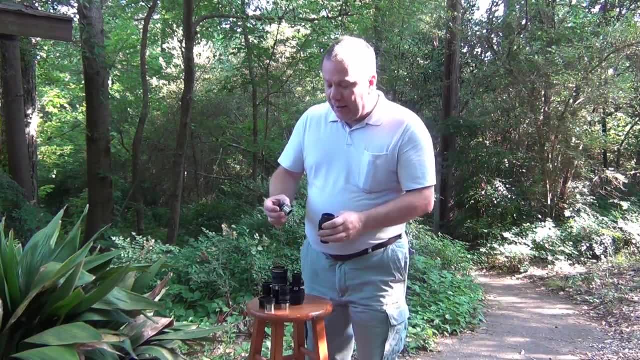 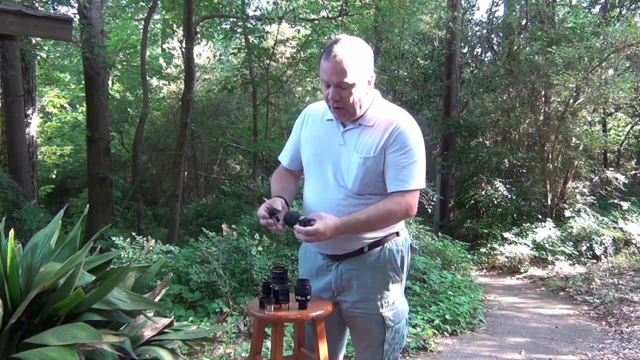 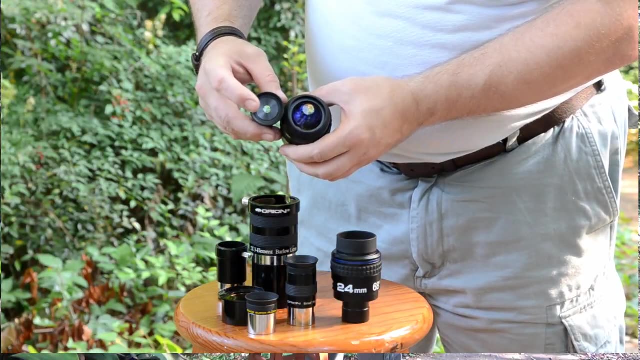 image ever used a high magnification, like, let's say, here's a 10 millimeter and here is a 13 millimeter. so they're reasonably close. look at the size of the glass on that one versus this one. you notice this is teeny tiny and that's quite big. the difference here is that i can get my eye. 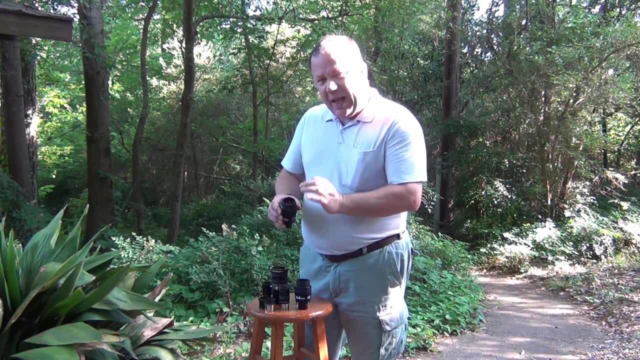 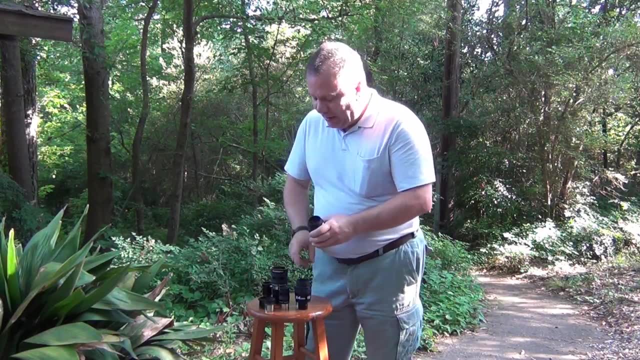 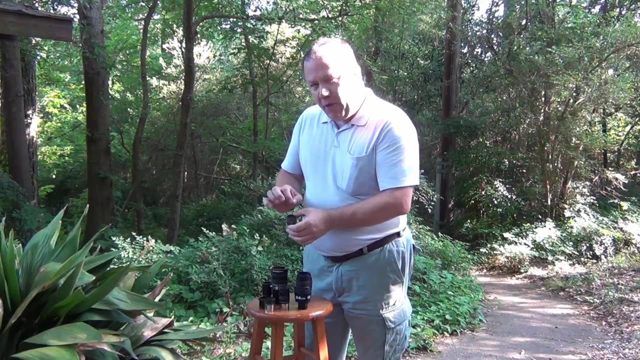 anywhere near this glass right here and the image is still in in focus. if i'm a little over to the sides, that's fine. if i'm a little far back or a little close, that's fine. with the smaller ones, with the tinier glass in here, your eye needs to be perfectly centered and it's almost difficult. 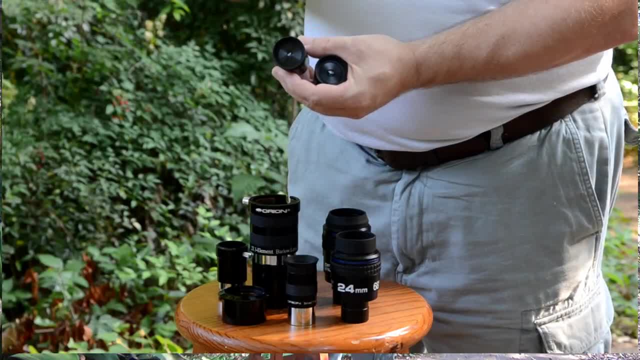 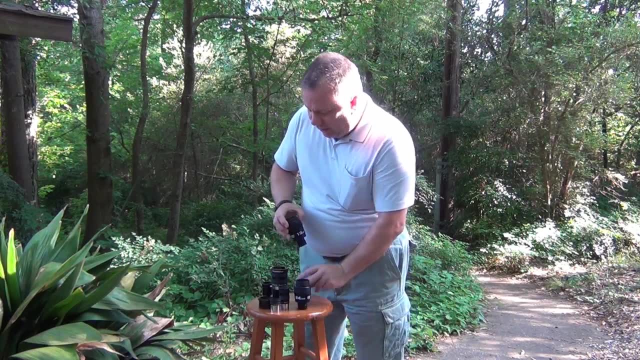 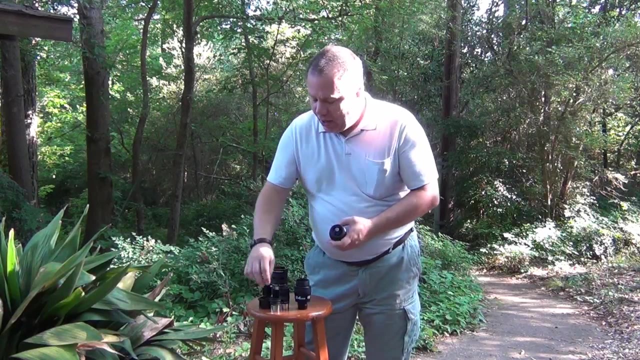 especially when you get down into, like this, 6.4, is incredibly hard to get your eye perfectly centered over it so that you can get a good image. these that have the larger glass in them- easy, very easy. and it's not just easy. With these smaller ones, it's almost impossible to be able to get a good image. 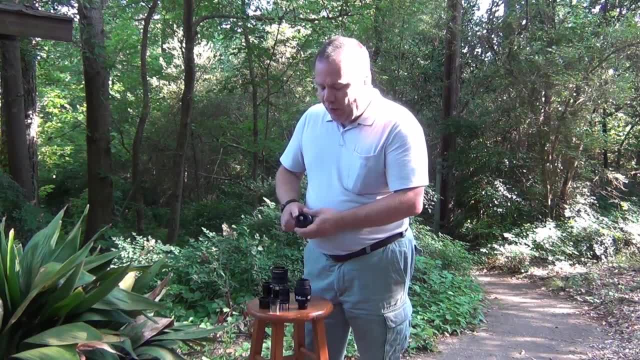 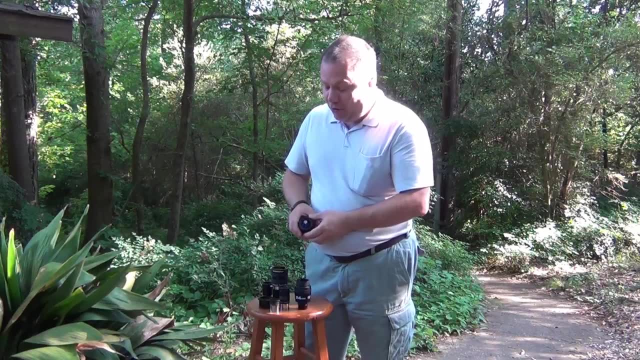 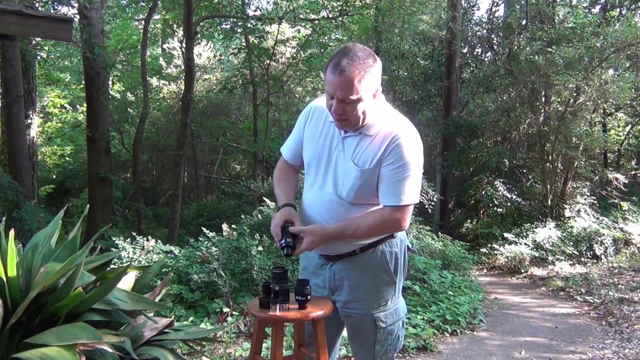 if you wear glasses With these larger ones, they have enough eye relief that you can wear glasses, glasses and contacts, bifocals, pretty much anything, and you're okay. The next thing to worry about is field of view. Field of view in this case. on these is printed right here: 68 degrees. 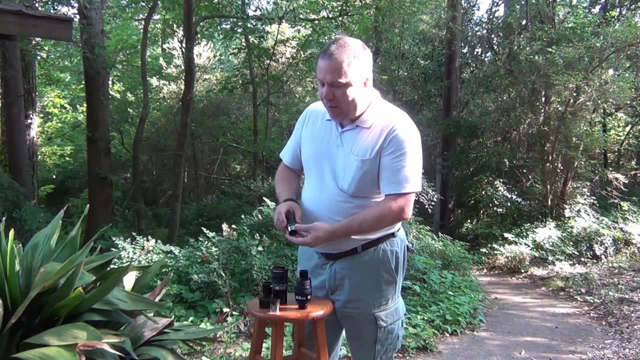 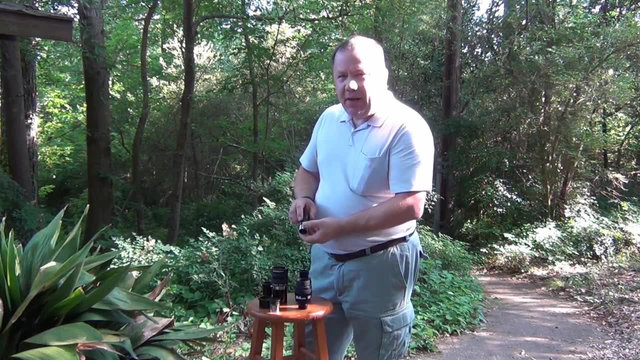 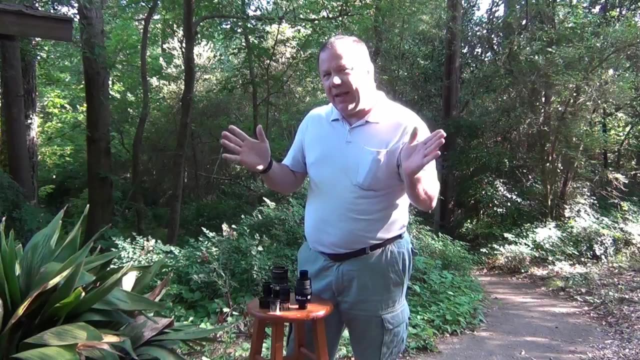 The smaller ones. you can go anywhere, depending on the quality of the eyepiece and the design, from 40 to maybe 50 degrees in eye relief. Now, what that is is how wide your field of view is how much of the sky you see at the given magnification. So that number the bigger. 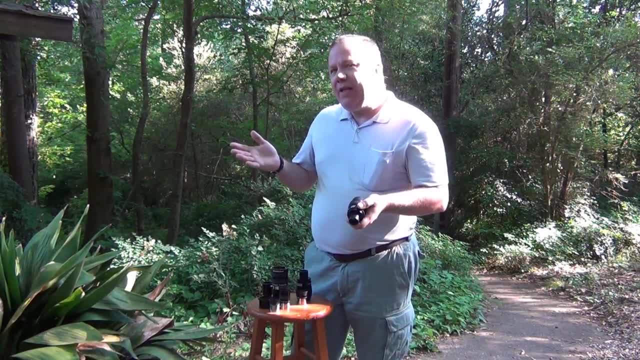 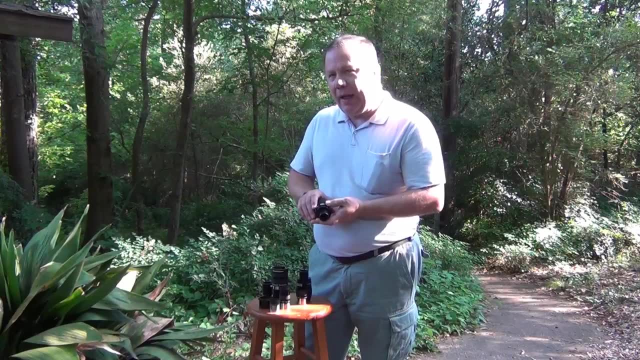 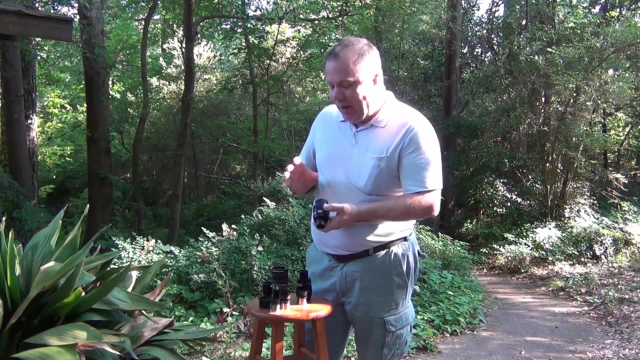 this number is the more of a walking in space feel you'll get. Personally, 68 degrees is kind of the minimum that I really like. 80 is kind of the maximum. Anything over 80 stuff just kind of gets lost for me. but that's personal preference. Some people really like the. 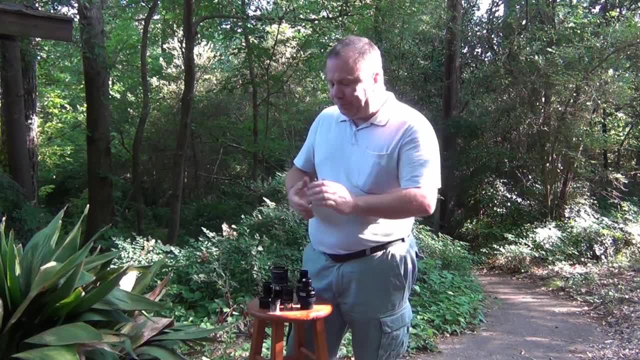 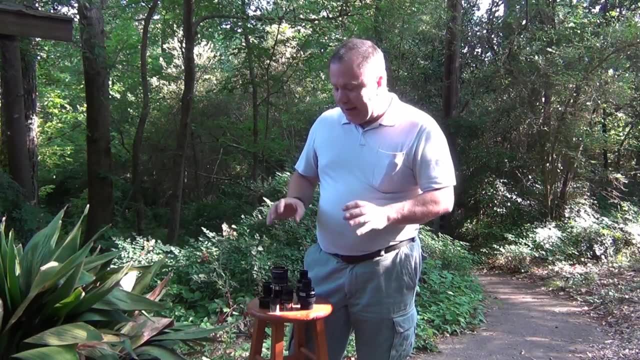 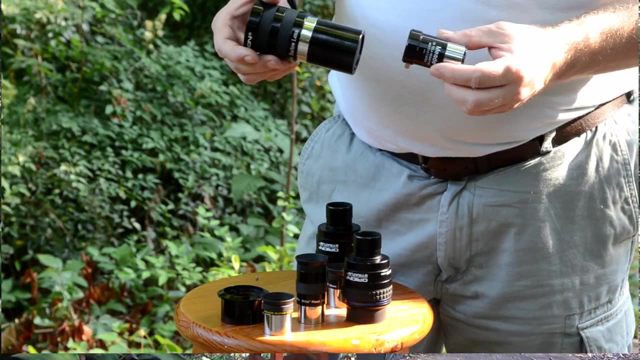 smaller field of view of these small eyepieces, and that's okay. Now another problem we have is we don't want to buy too many eyepieces, so a lot of telescope manufacturers include what's called X-barlows. This is two different kinds of barlows: A two-inch barlow and a smaller inch and a quarter. 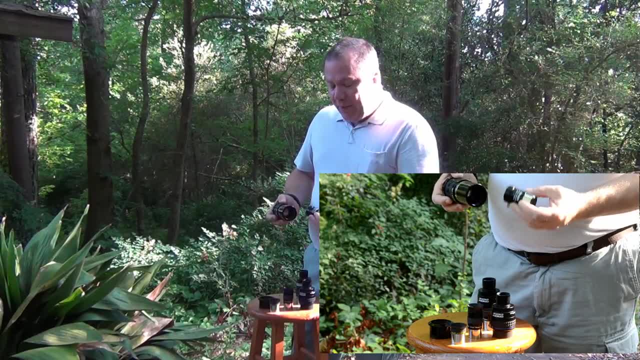 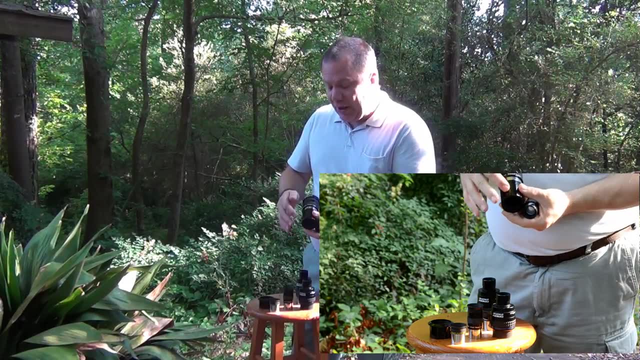 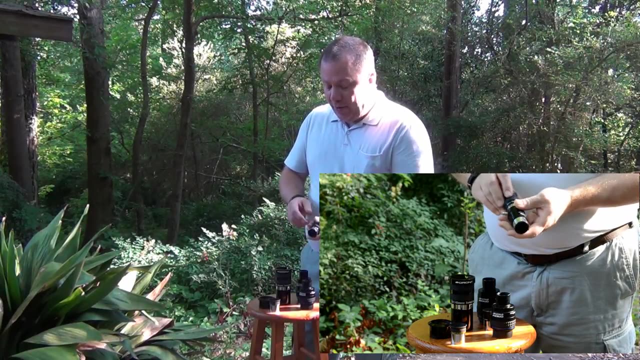 barlow. Now, both of these do basically the same job. Both of these are 2x barlows, meaning that if you put an eyepiece in this end and put this end in the telescope, it gives it twice the magnification. So if you have this 25 and you put it in here, we got 40 when we did the math: 40x magnification. 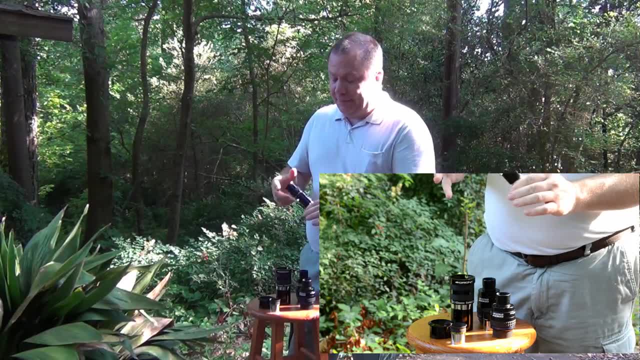 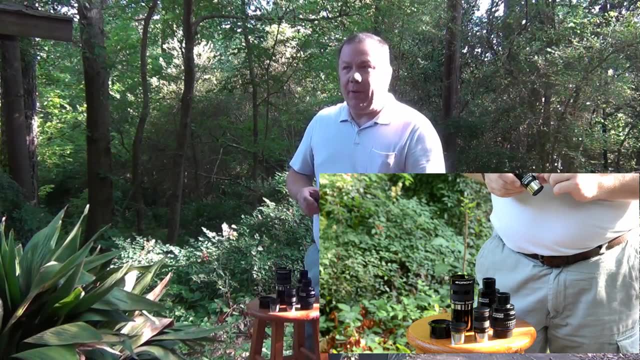 When you stick this in a telescope like that, you're going to get 80.. Now, barlows not only double the magnification- assuming you get a 2x barlow, and they come in 1.5s and 2s and 3s- but they also 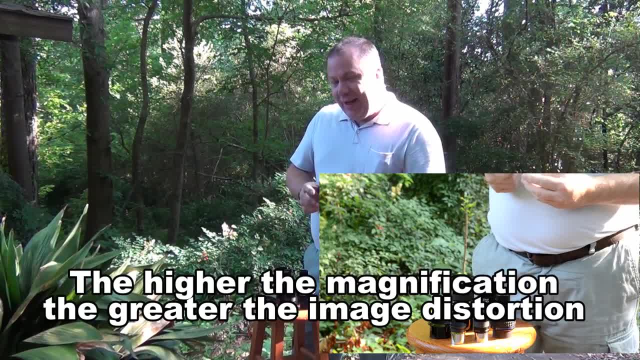 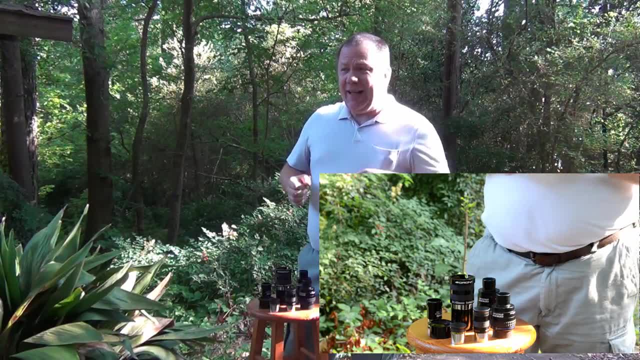 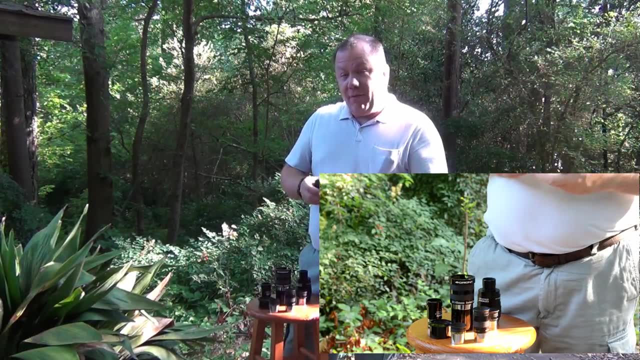 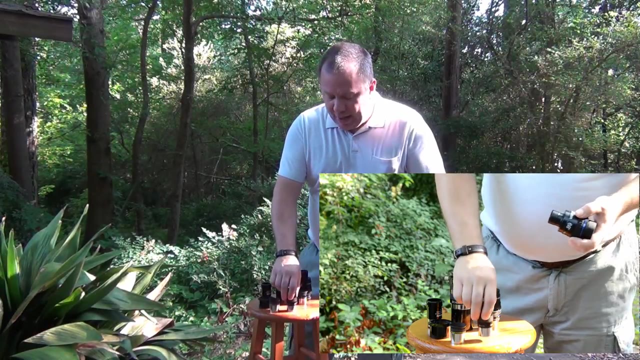 degrade the image slightly, But they are a very inexpensive way to round out your eyepiece collection. Now, the quality of the eyepiece, number of elements, the coatings on it, all of that affects it. Now, eyepieces like this cost $150 and eyepieces like this cost $30. And you can get. eyepieces that go up into $600, $700, $800, $900 a piece. Is it worth it? Well, on the high-end telescopes, after you've had years and years of experience, possibly, For me not really Anything. over $300 or so for an eyepiece is expensive. 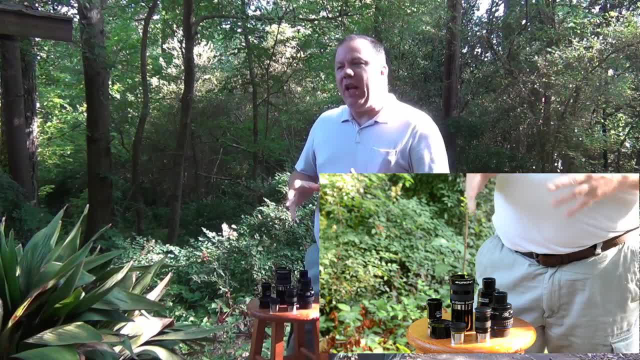 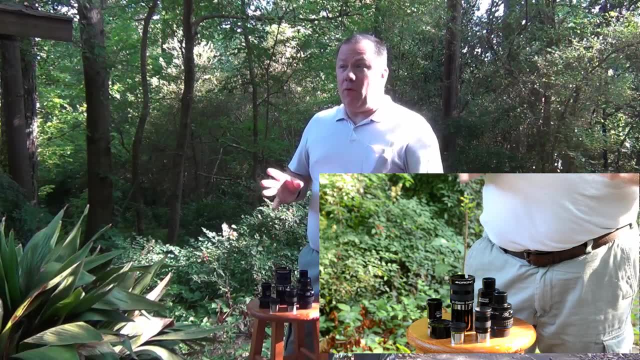 And it's just not. I don't get enough out of it. Now you notice I'm saying $300 or so and you may be thinking, oh my god, you know I want 10 eyepieces, and at $300 a piece. No, you don't want 10 eyepieces. 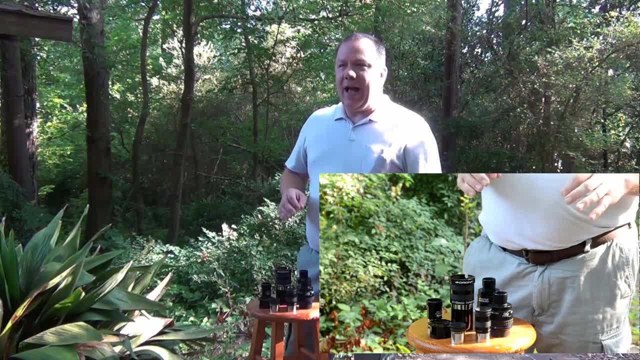 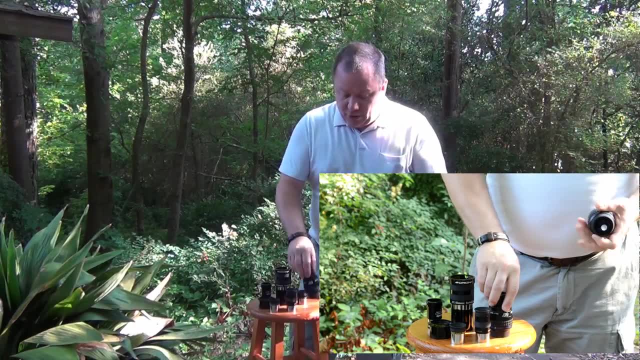 When I go out into the field, generally speaking, I carry four eyepieces, and if I use more than two, something special is going on. The two that I use the most are right here. It's a 24 millimeter and a 13 millimeter, And not a lot of eyepieces, So I'm going to go ahead and take a look at this one. 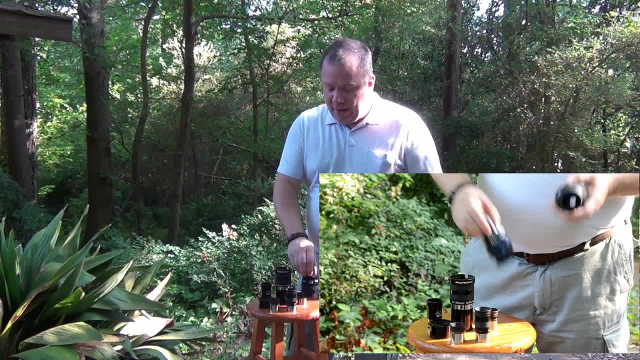 And I'm going to go ahead and take a look at this one, And I'm going to go ahead and take a look at this one. 90% of my viewing is done with these two eyepieces. On very rare occasions I will grab a. 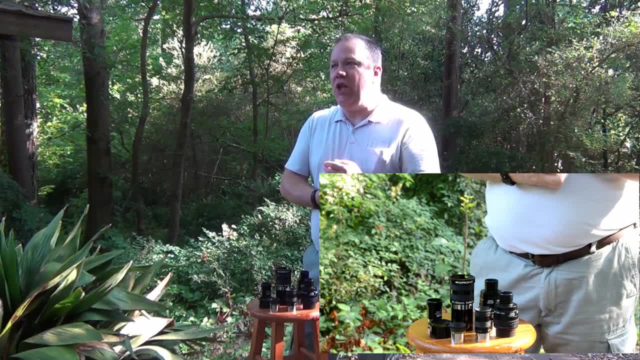 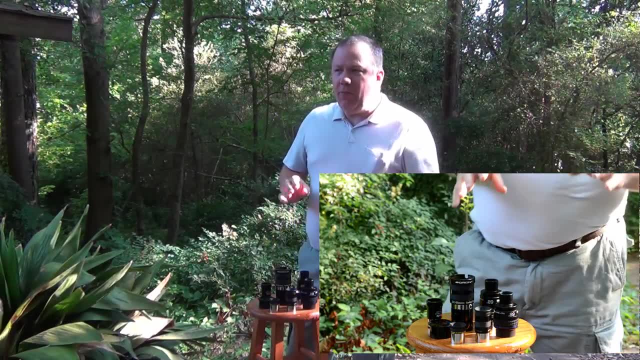 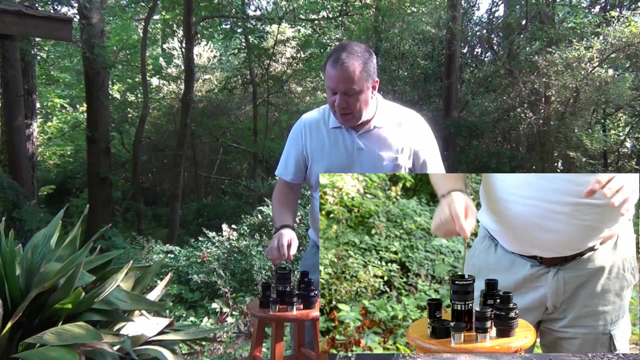 smaller eyepiece. I have an 8 that I get to use- maybe I don't know- twice a year if I'm lucky. So you really only need a couple of really nice eyepieces. I highly recommend with beginner telescopes that you get something like a 25 and maybe a 15.. So if your telescope already came with 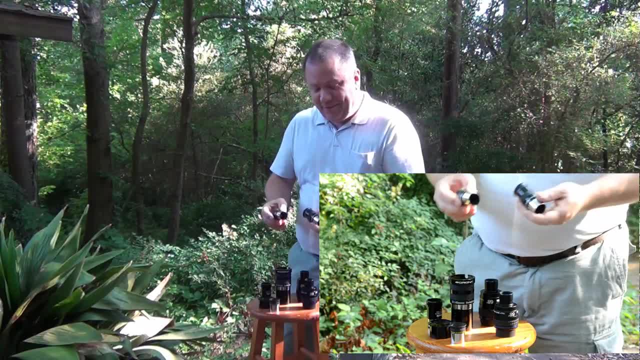 a 25 and you're going to need a 25 and you're going to need a 25 and you're going to need a 10. if I can find it, The next eyepiece I suggest you get is right in between the two, pretty much. Get like a 15. And you don't have to spend a lot of money on it. Get you a 15 like this little serious, and you'll probably spend anywhere from 30 to 50 dollars for one new And that's fine. 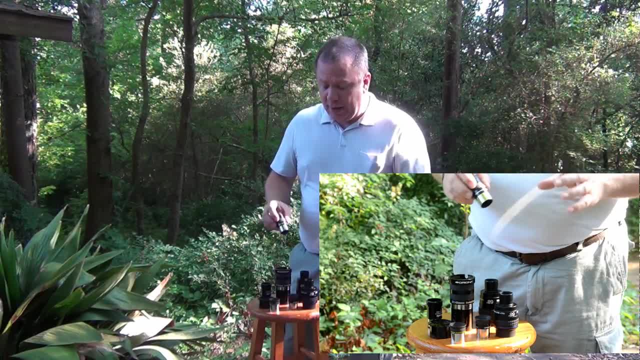 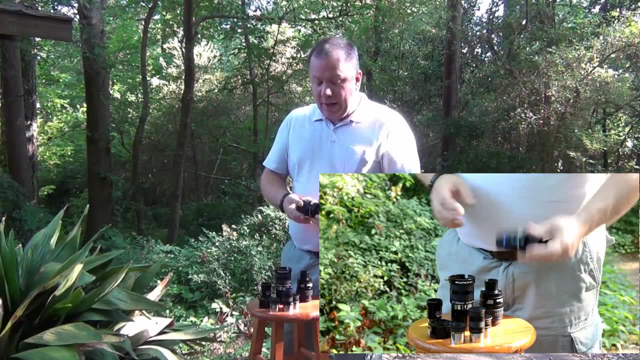 Now you've got plenty of eyepieces and plenty of magnifications to do what you need to do. If, then, you want to step up and get something much, much, much nicer, you can look at something like these Orion Stratuses. Now Bader Hyperions are a. 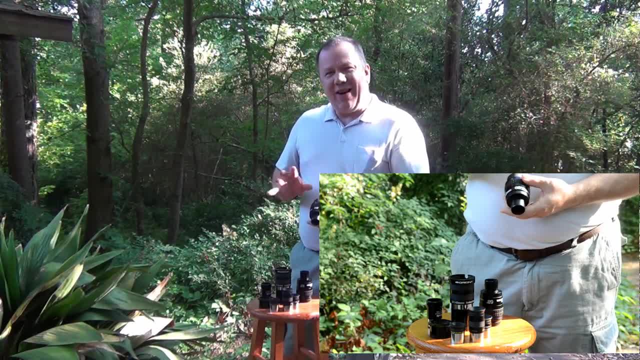 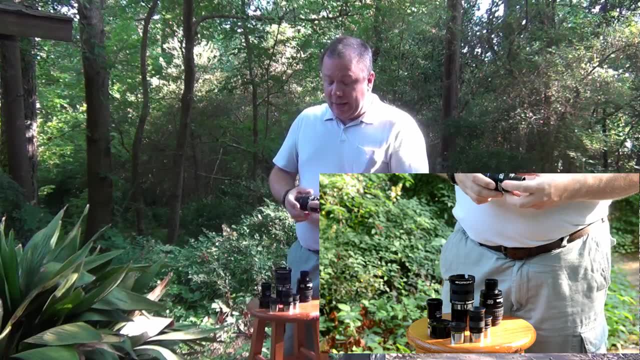 very similar model. They're probably made at the same plant. Whether or not they're identical I don't know, but they're extremely close. So the Orion Stratus or the Bader Hyperions are both nice. They're nice because they'll fit the smaller and the larger eyepieces, So no matter what your 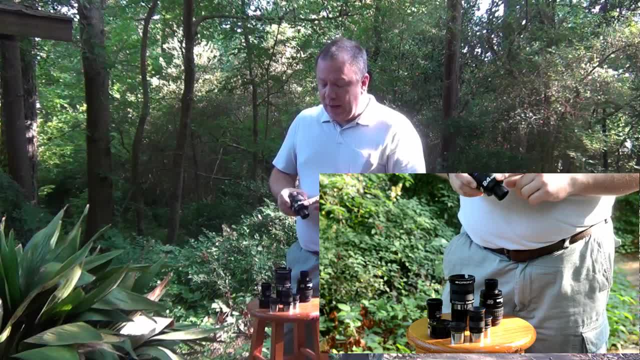 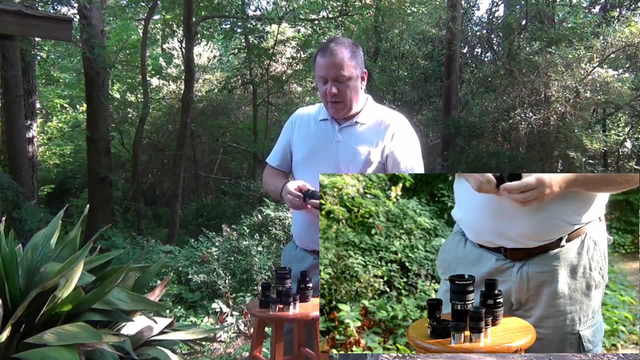 telescope uses. whether it's the inch and a quarter or the two inch, they'll fit just fine. They've got plenty of eye relief. They're hefty enough that you're not going to let them slip out of your hand. They've got nice rubber grips on them. 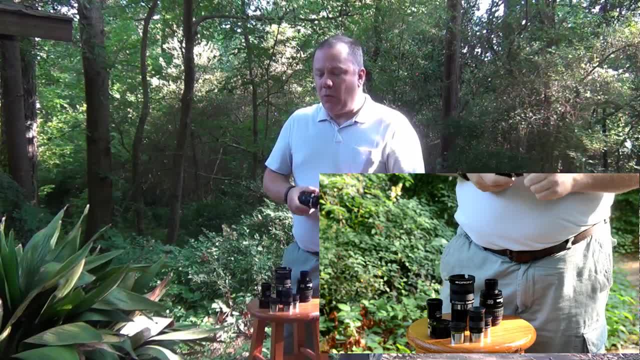 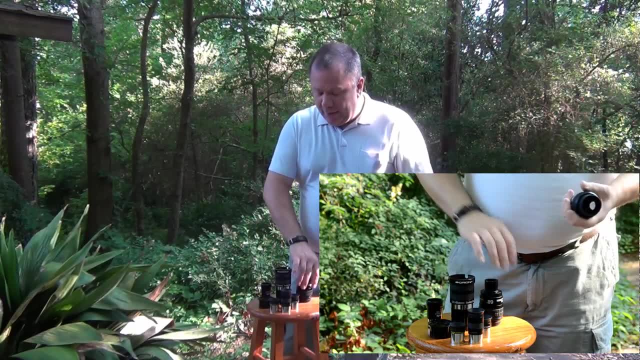 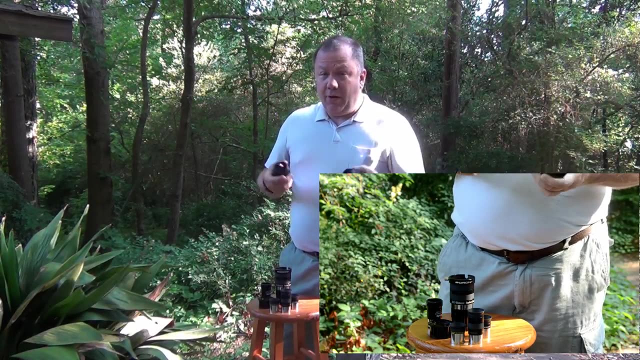 They've got a good field of view And price wise. you know for what you pay for two or three of these. you can get one of these, And if you only need two, then you're done, Because even if you paid full price for these, which I think is about $150 each, that's $300. And you've got.